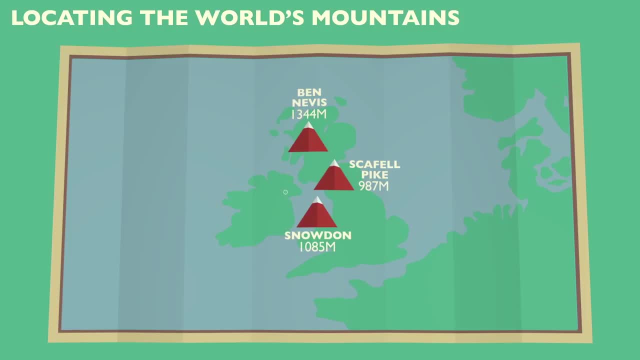 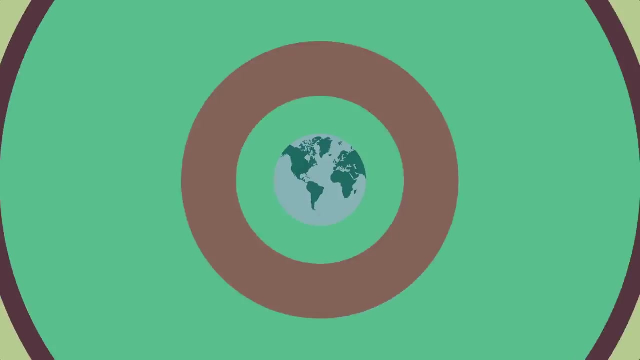 at a height of 987 metres and Sleave Donard in Northern Ireland at 850 metres. So we know where the significant mountains are located, but the question remains: how exactly are they formed? To understand how mountains are formed, we first need to take a closer look at the structure. 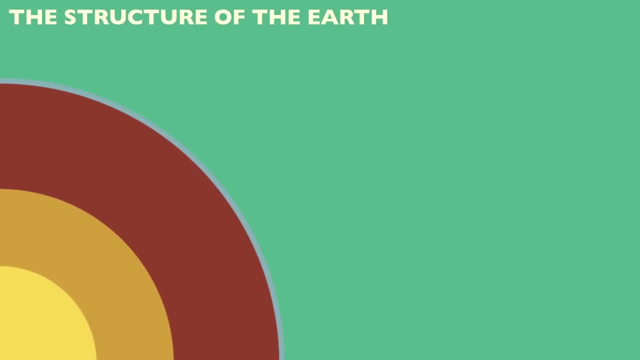 of the earth. The earth comprises of four main layers. The inner core is a solid ball of iron With a temperature of 5,500°C. it is almost as hot as the surface of the sun, Sharing a similar temperature. the outer core is a liquid layer composed of iron and nickel. 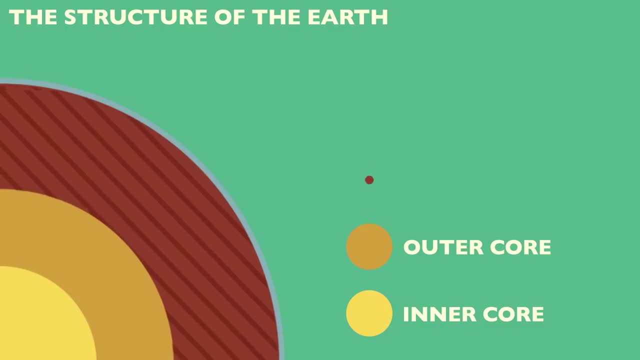 Next, with a depth of 2,900 kilometres, the mantle is the thickest layer. The mantle is a viscous mix of semi-molten rock or magma, Not quite a solid and not quite a liquid. The magma is also extremely hot. 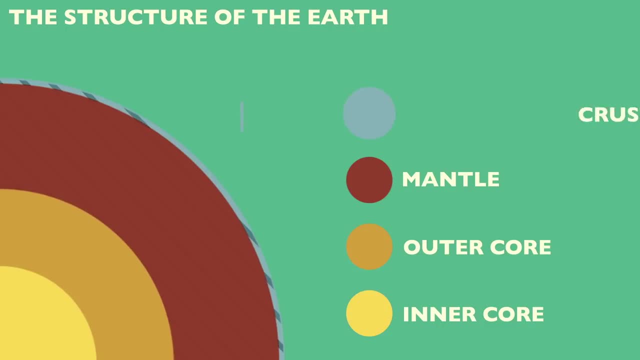 Finally, resting on top of the mantle, is the crust, Composed of solid rock. the crust is the outer layer of the earth's surface, Between 0 and 60 kilometres deep. it is the thinnest of all the layers In terms of depth. think of the earth's crust as the skin of a tomato, not the peel. 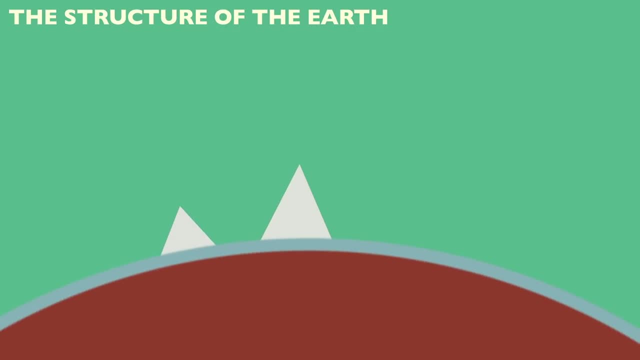 of an orange. It is in the crust that our mountains and other features of our landscape are formed. The earth is a solid rock. The crust is the outer layer of the earth's surface. Between 0 and 60 kilometres deep, it is the thinnest of all the layers. 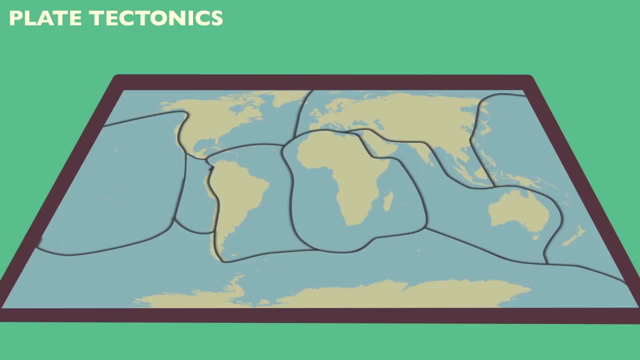 The earth's crust is not one smooth, unbroken covering. rather, it is made up of different sections called plates. There are eight major plates: The Eurasian, African, Indo-Australian, Pacific, North American, South America, Nazca and Antarctic. 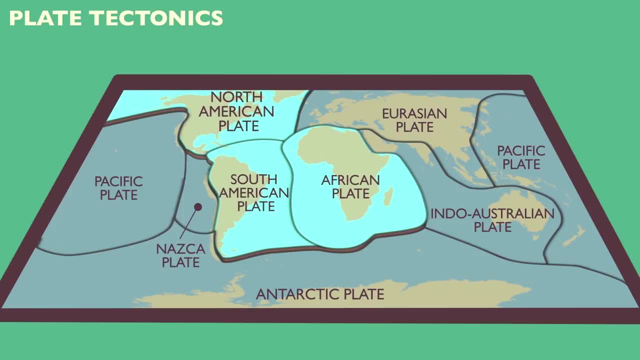 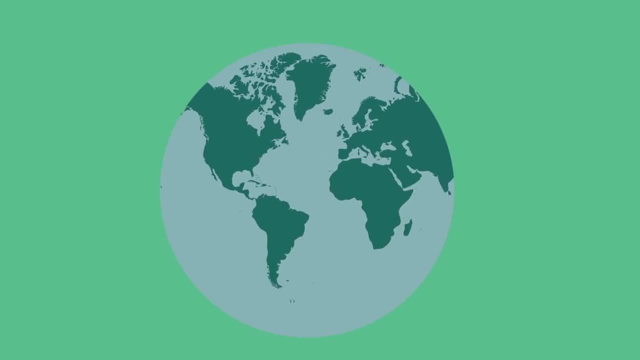 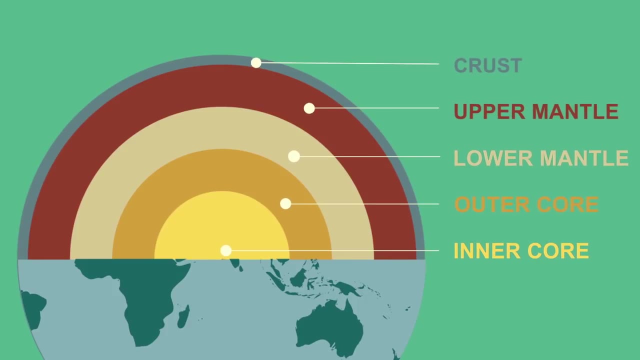 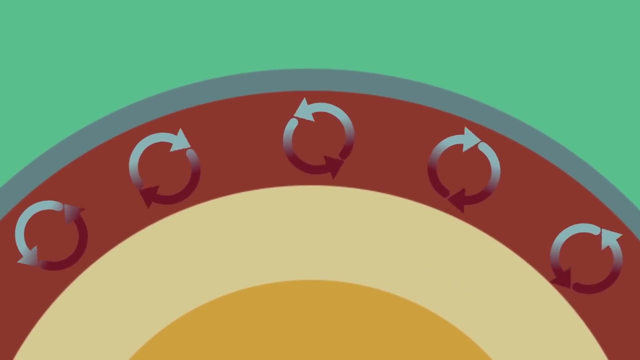 Some plates mark the boundaries of continents. Other plate include more than one politically defined continent. The earth's plates are constantly moving. On average, this movement is between 1 and 10 centimetres each year. Within the mantle, heat rises and falls throughout the molten rocks. 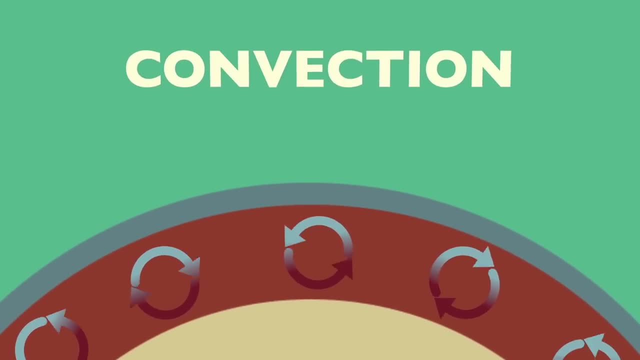 This causes convection currents, CONVICTION, CURRENCY CONDITIONS, BITTERNESS AND LIGHTENING convection currents: as the magma moves, so do the plates above the movement of the earth's plates, and the changes this causes is called plate tectonics. the theory of plate tectonics explains. 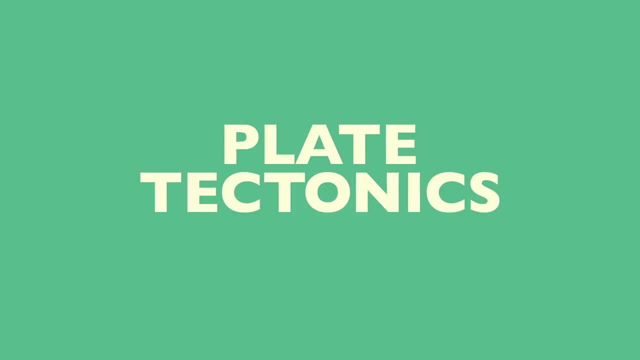 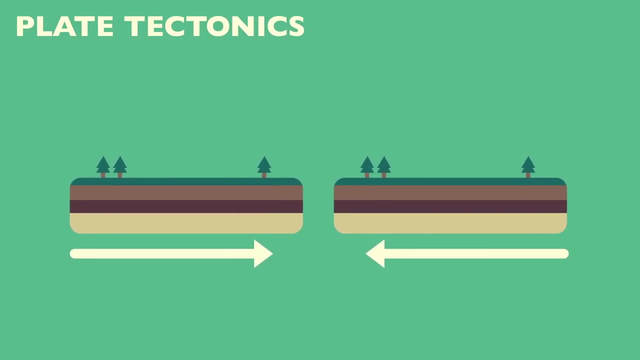 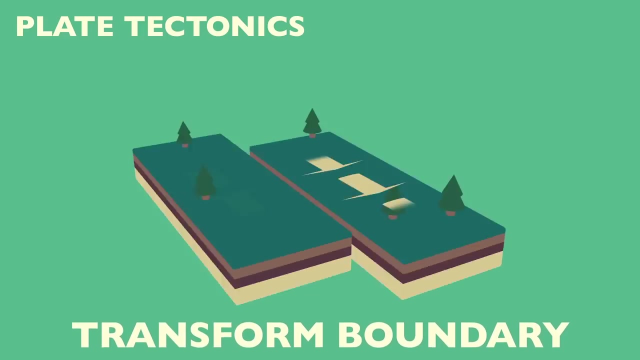 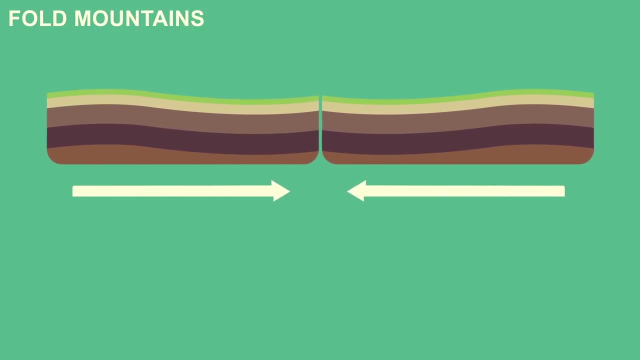 how mountains are formed and why volcanoes and earthquakes occur. plates can move in different ways. they can move towards each other or converge. they can move away from each other or divert. plates can also move in parallel along a transform boundary. as two plates move closer to each other or converge, this creates intense pressure. this pressure can 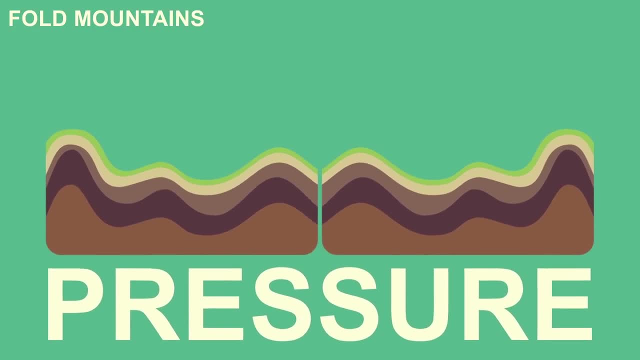 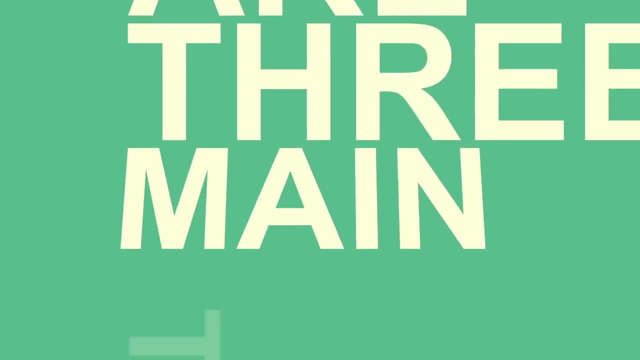 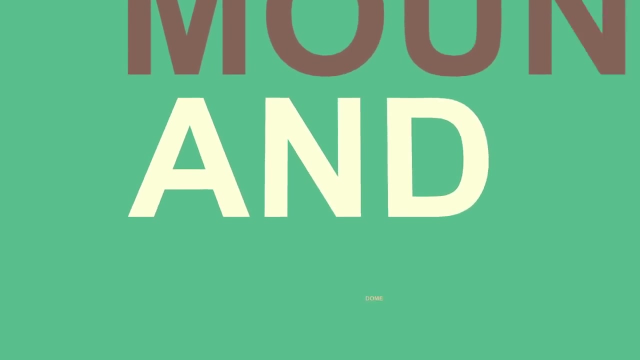 cause the plates to buckle in different ways. This process over millions of years can form a mountain. There are three main types of mountain: fold mountains, fault block mountains and dome mountains. Fold mountains are the most common type of mountain as two plates. 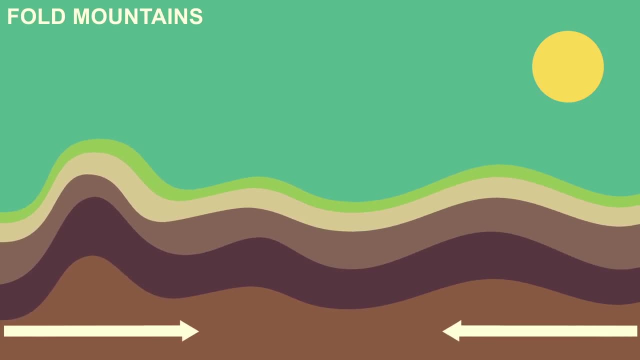 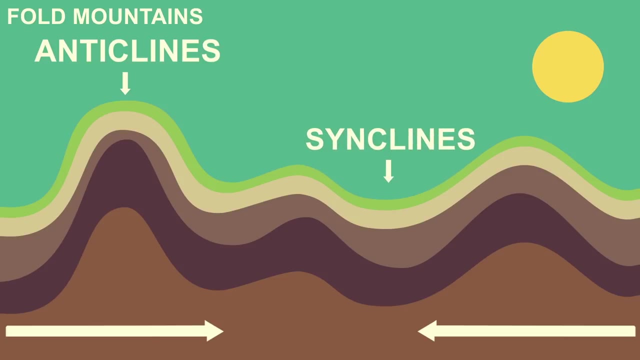 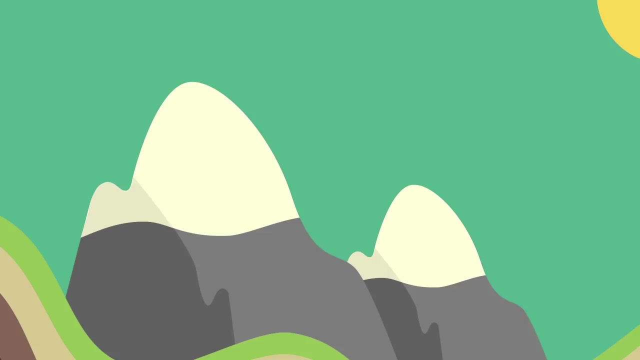 converge, the crest pushes upwards, forming the upwards folds, or anticlines, and the downwards folds, or synclines, of the mountain Fold mountains are, geologically speaking, relatively young, For example, Mount Everest, among the other peaks of the Himalayan mountain. 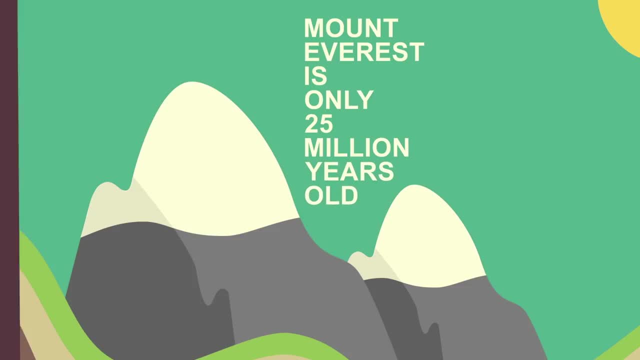 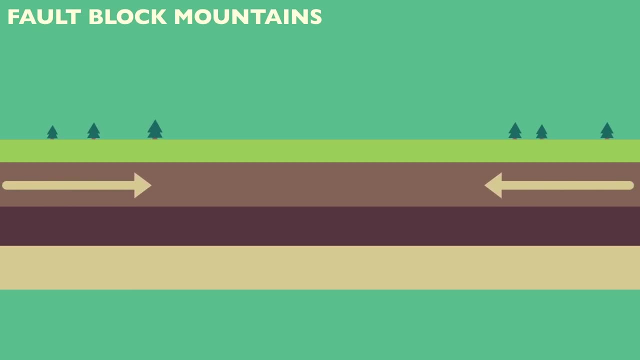 range was formed only 25 million years ago. Fault block mountains are also formed when two plates converge. Rather than the crust folding under the intense pressure of the moving plates, it cracks along lines of weakness called fault lines. The crust then breaks into a block which is pushed. 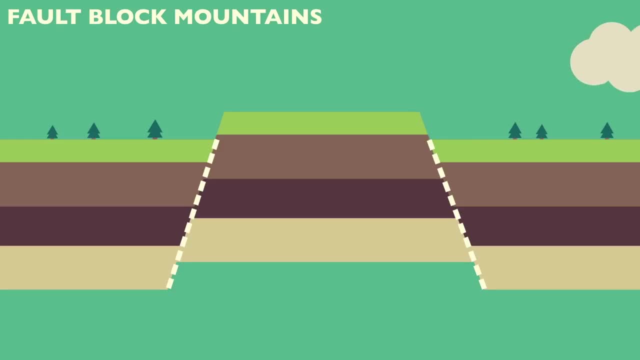 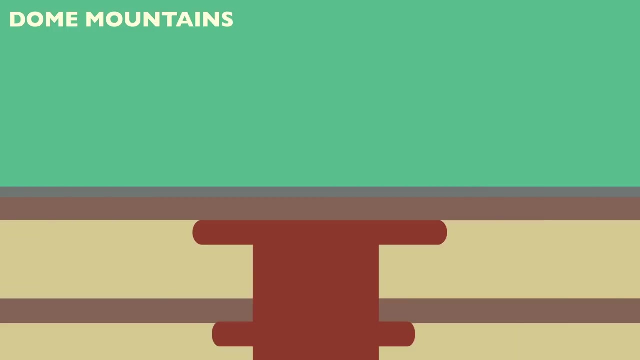 upwards. The action of the wind and rain through the process of weathering and erosion will also help to shape the mountain. In some cases, the block in between the fault lines is pushed down to form a rift. valley Dome mountains are the result of molten rock from the mantle pushing its way up under 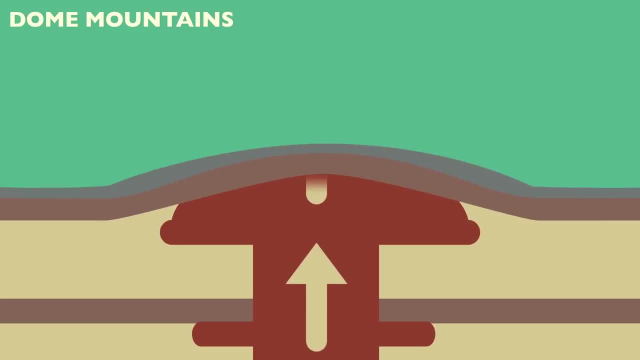 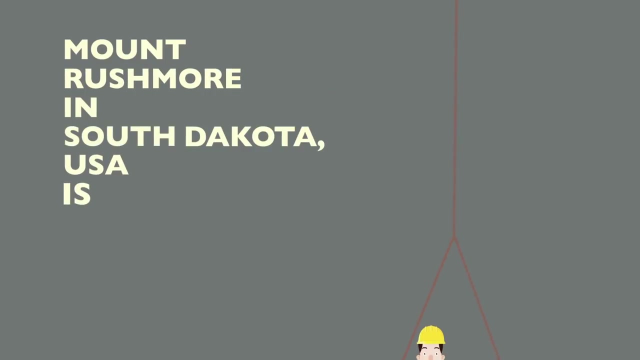 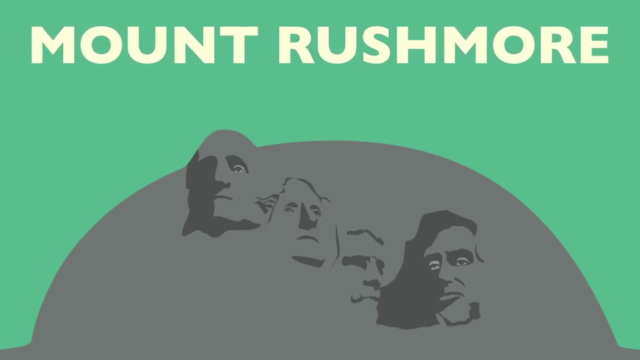 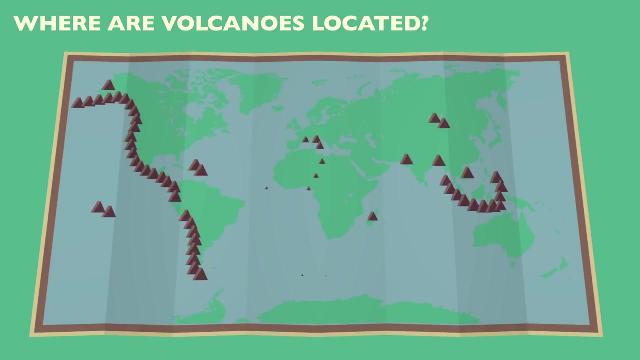 the earth's crust Without actually erupting onto the surface. the magma pushes up the overlaying layers of rock, which then bulge upwards. Eventually, the magma cools and becomes hardened rock. There are approximately 500 active volcanoes in the world. On average, 25 of these erupt each year. 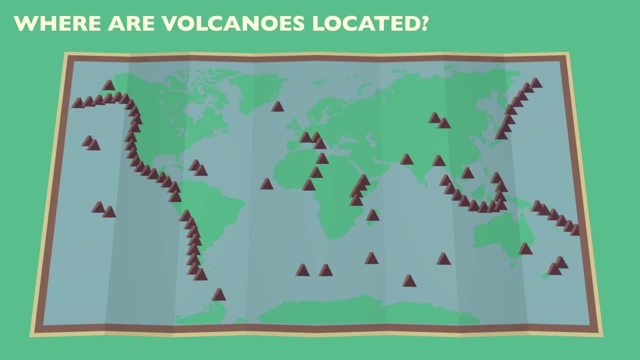 Volcanoes, like earthquakes, primarily occur on the boundary between two tectonic plates. Volcanoes are formed when magma penetrates through the earth's crust. Some volcanos are active, erupting regularly. Other volcanoes, such as Bajax, the, 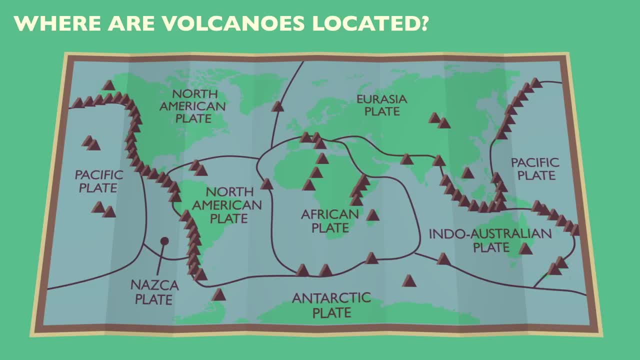 Olympic volcano may also fall apart: The Poke Volcano. Thank you for watching. You're welcome. imaginingebangland, là. Hey there. You've learnt something new today Which, over the last unc adulthood, your mind has changed. Crног damage is a sign of through the crust This isorge on a volcano's crust. It might be happening that rock land Deus has been erupting regularly before. 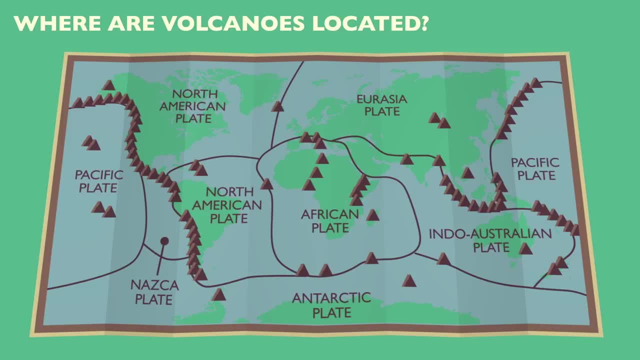 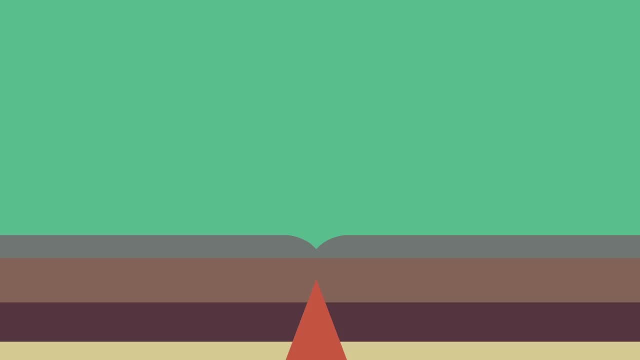 Others are dormant and have not erupted in the recent past. Extinct volcanoes are dead and will not erupt again. At constructive plate boundaries, tectonic plates diverge or move apart from one another. As they move apart, molten rock rises or erupts from the mantle before cooling and hardening into solid rock. 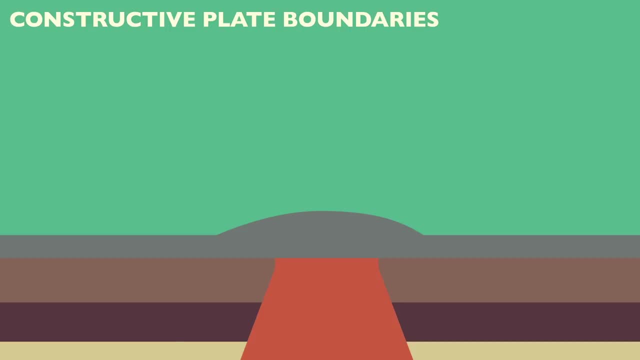 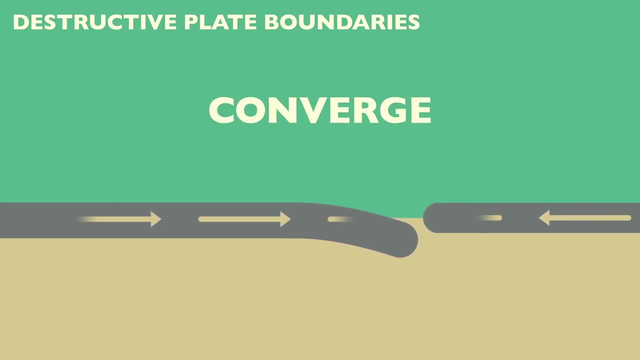 At destructive plate boundaries. tectonic plates move towards one another or converge. As the plates meet, one plate is pushed underneath the other lighter plate. The point at which the one plate is forced beneath the other is called the subduction zone. 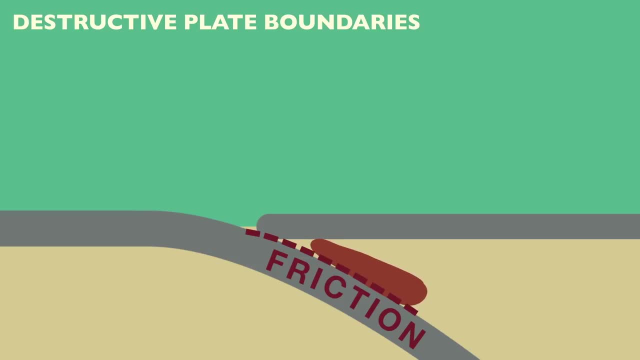 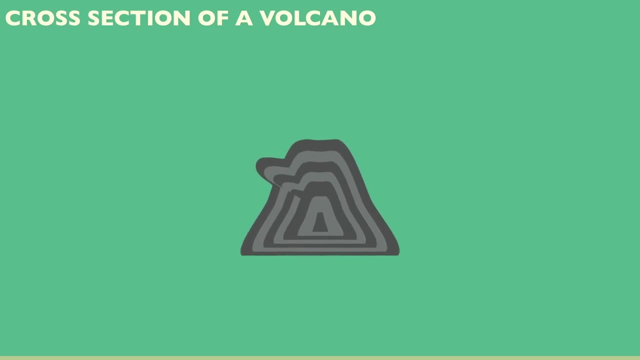 Friction causes the plate to melt, becoming molten magma. The magma then forces its way up the side of the plate. The magma then moves up the plate boundary to form a volcano. One of the key features of a volcano is the magma chamber. 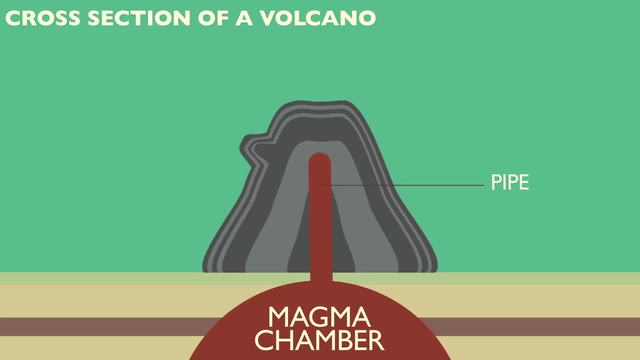 From this, the magma rises through the pipe or central vent to the surface, forming lava. Eruptions take place through the crater and are accompanied by a toxic cloud of gas, ash and rock particles, together called pyroclastic flow. Over many eruptions, layers of lava and ash build up. 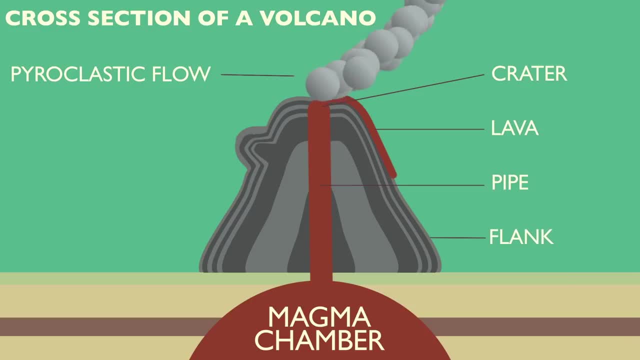 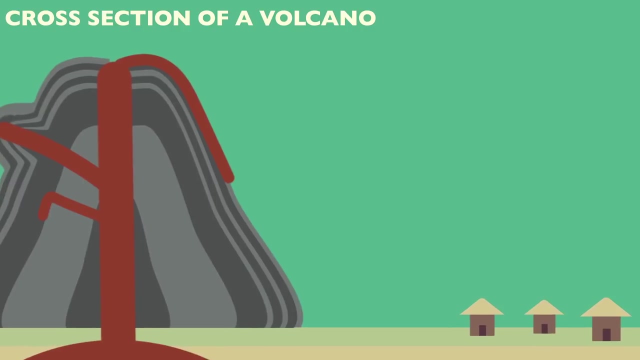 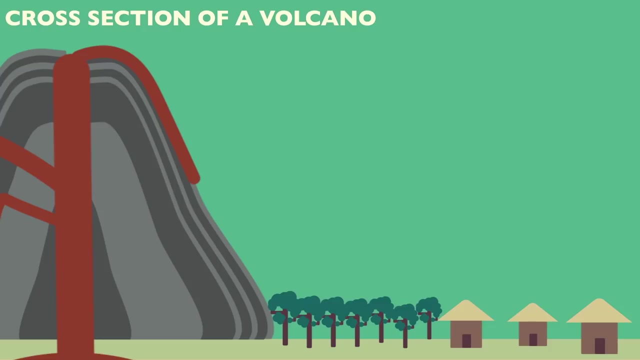 forming the flank of the volcano. Occasionally, branch, pipes, sills and parasitic cones are formed. The land around a volcano is rich in minerals, resulting in fertile soils ideal for agriculture, But living in the vicinity of a volcano can be very dangerous. 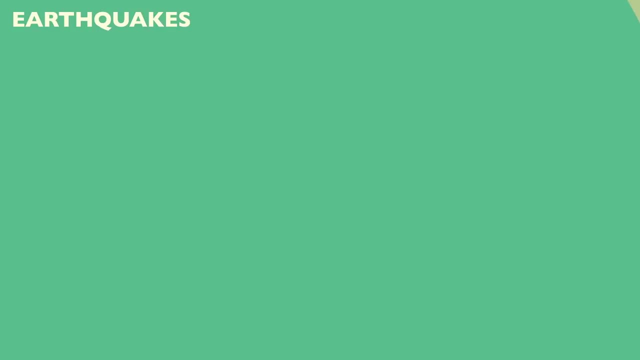 This is why it is important to keep a close eye on the volcano's surface. It is also important to keep a close eye on the volcano's surface. Every 30 seconds there is an earthquake somewhere in the world. Earthquakes are common at transformed plate boundaries. 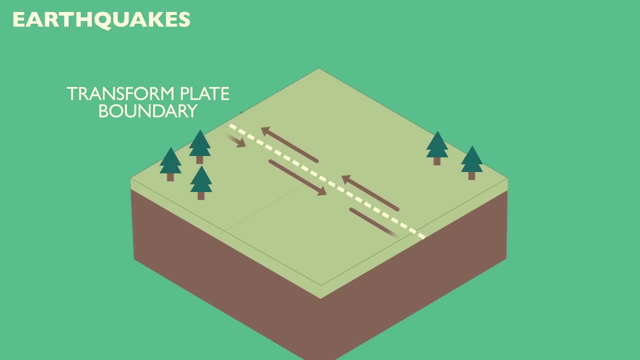 As two tectonic plates move in parallel, friction causes them to stick. When they eventually become unstuck, it is often with a violent jolt. This jolt causes an earthquake. The focus of an earthquake is the point deep underground where the earthquake begins. 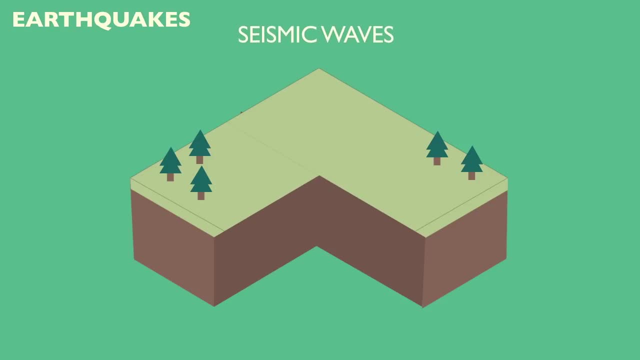 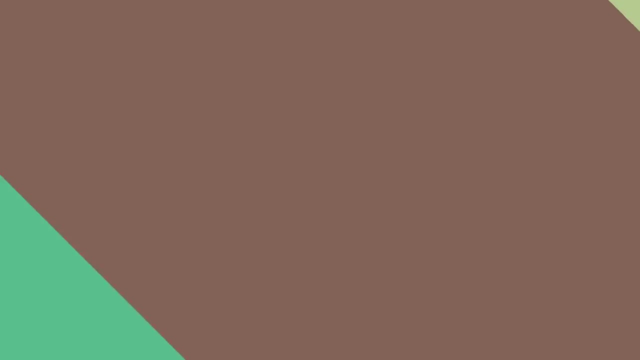 When the earthquake is triggered, shockwaves, called seismic waves, spread out in all directions from the focus. The epicentre is the point on the Earth's surface immediately above the focus. It is here that the earthquake is felt most strongly. Earthquakes have different strengths or magnitudes. 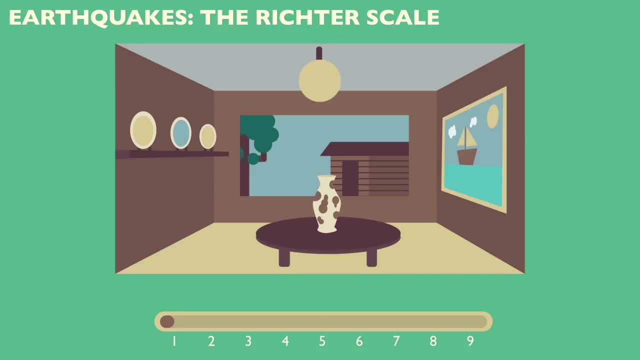 While some earthquakes are barely detectable, others can cause severe damage to property and result in terrible loss of life. The Richter scale measures the magnitude of an earthquake. Earthquakes with a magnitude of 3 are the smallest commonly felt by people, but cause no damage. 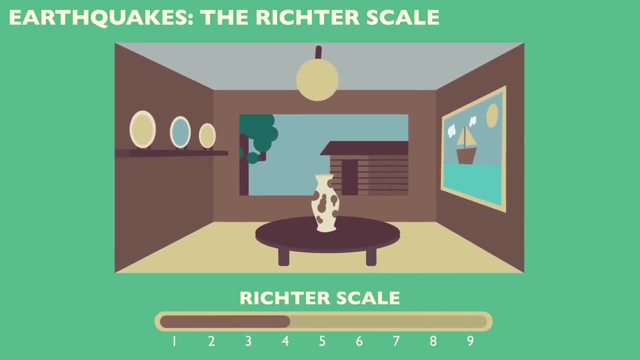 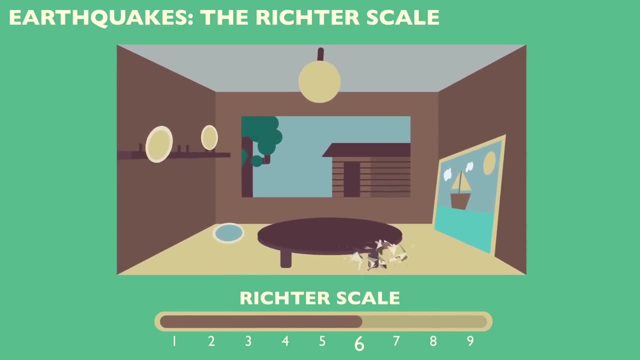 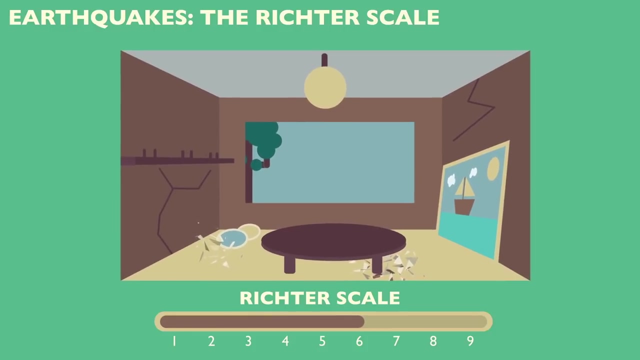 With a magnitude of 4, an earthquake can make windows rattle and there may be some minor breakages. With a magnitude of 6, there will be serious damage, Walls crack and split and buildings can collapse. With a magnitude of 9,, an earthquake is a severe, often catastrophic event. In theory, there is no upper limit to the Richter scale.